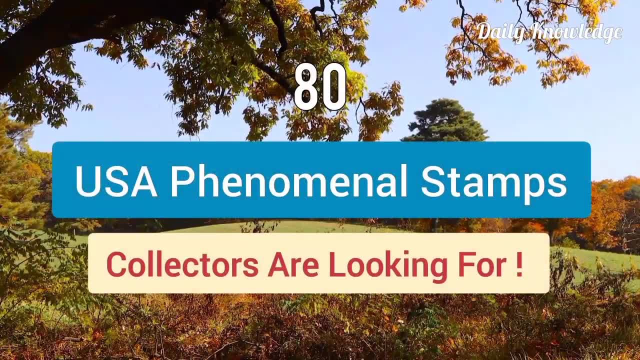 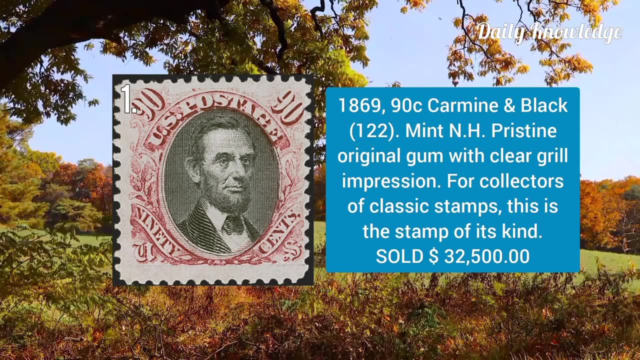 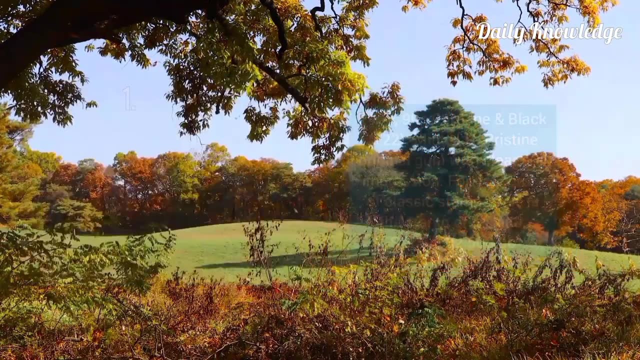 Hello friends, welcome to daily knowledge. This video is about 80 USA phenomenal stamps collectors are looking for. The first is 1869, 90 cent, carmine and black. It is mint, never hinged and has pristine original gum with clear grill impression. Next is 1868, 3 cent rose z grill and. 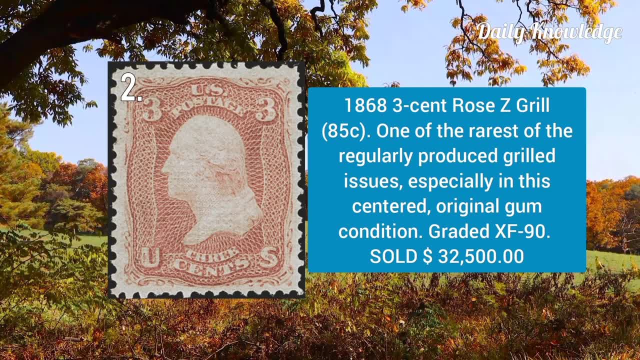 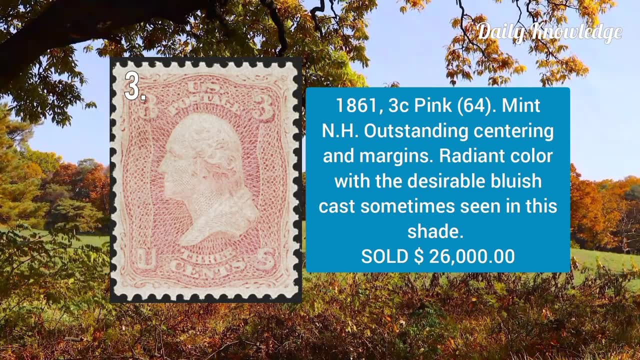 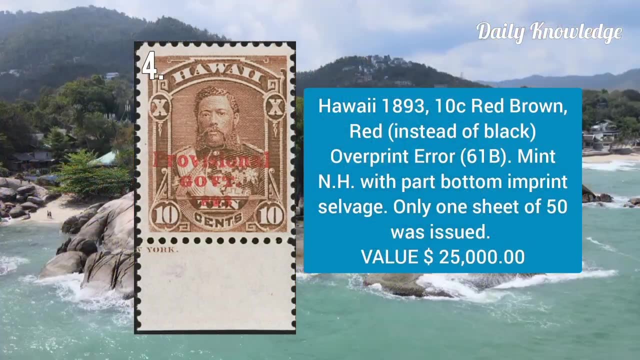 it is one of the rarest of the regularly produced grilled issue, especially in this well-centered original gum condition: 1861, 3c, pink mint, never hinged, outstanding centering and margins with radiant color. Next is from Hawaii, 1893, 10 cent red, brown, red instead of back over print error. 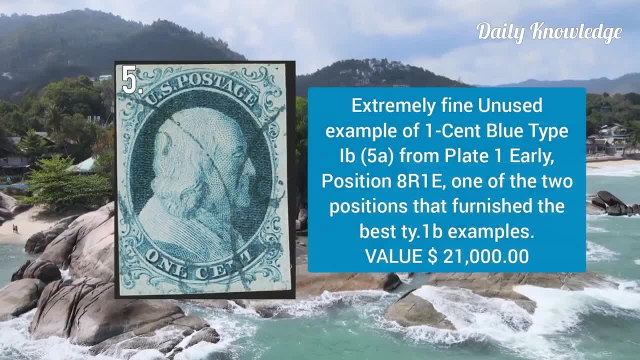 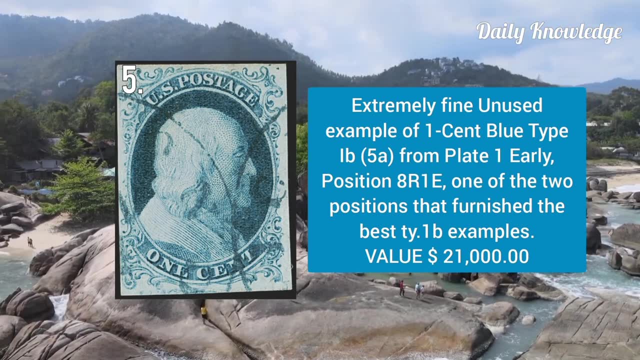 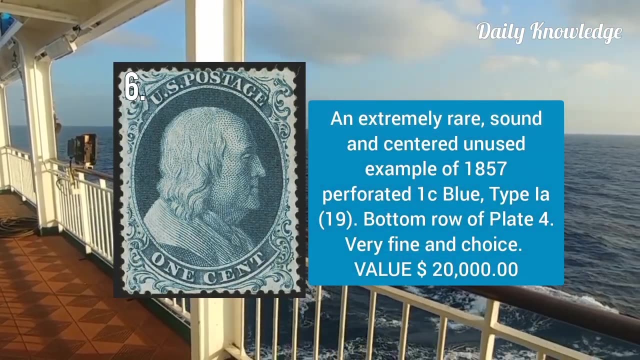 now it is mint, never hinged and only one sheet of 50 were produced. extremely fine, unused example of one cent blue type 1b and from plate one. it is early position. next is an extremely rare, sound and centered unused example of 1857 perforated one cent blue. 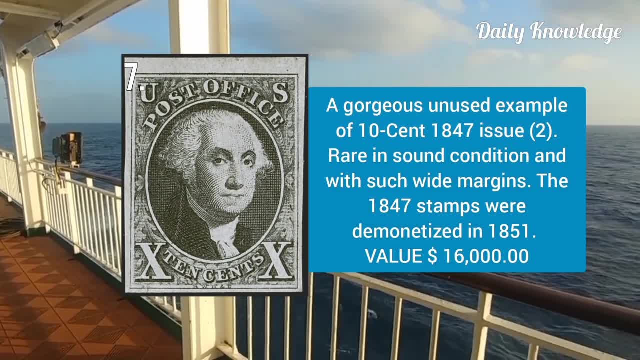 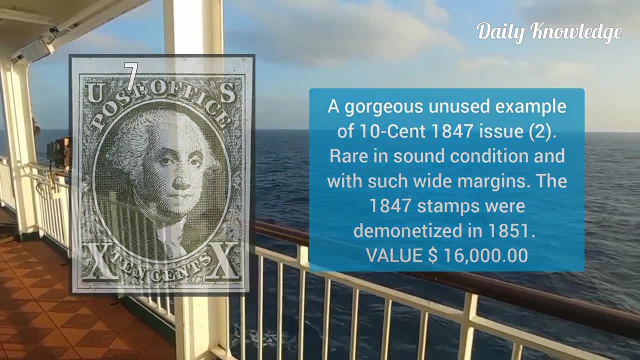 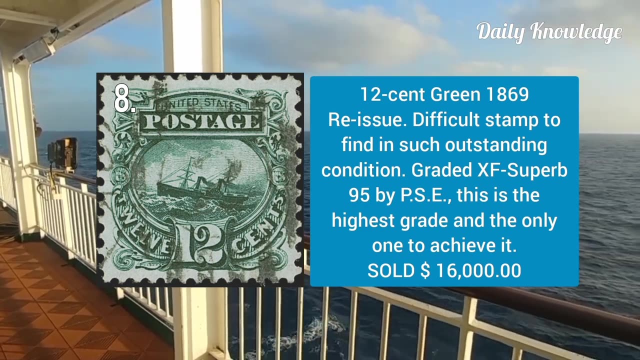 type 1a. now this is a gorgeous unused example of 10 cent 1847 issue. it is rare in sound condition and with such wide margins. next is 12 cent green 1869. it is a re-issue. it is a difficult stamp to find in such outstanding condition. next is a 12 cent green 1869. it is a re-issue. it is a difficult stamp to find in such outstanding condition. 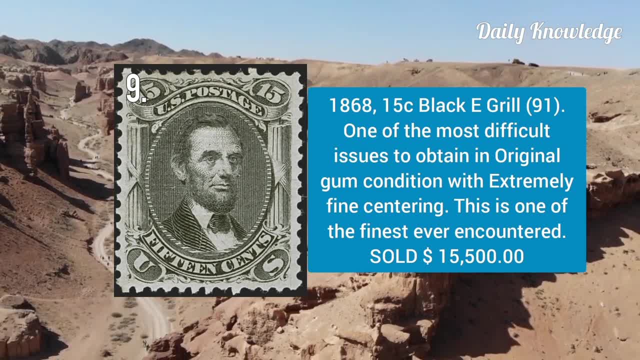 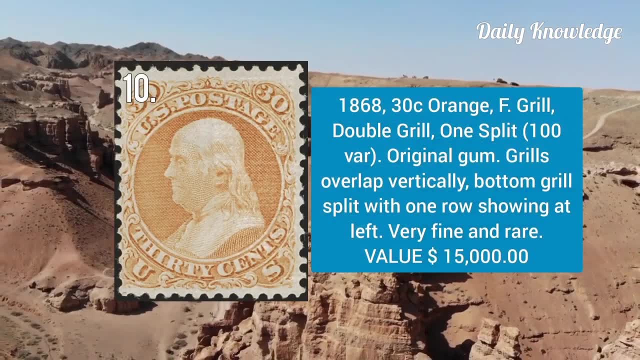 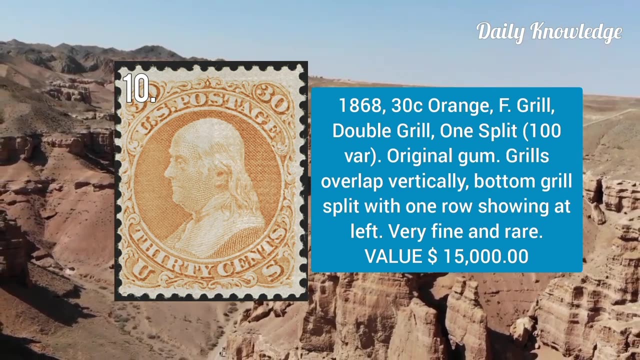 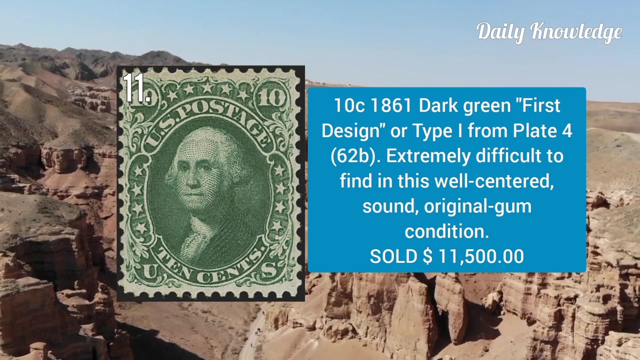 is 1868 15c black e grill. now it is one of the most difficult issue to obtain in the original gum condition. next is 1868 30 cent orange f double grill. one is split and it has original gum. it is very fine and rare. next is 10c, 1861, deep green, first design or type 1 from plate 4. it is extremely 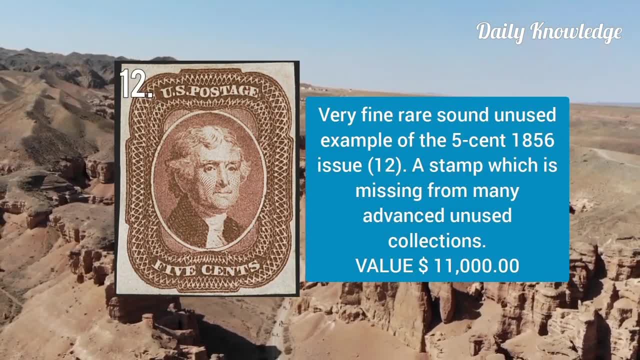 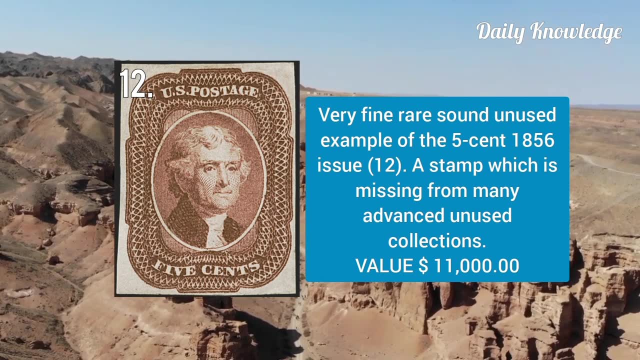 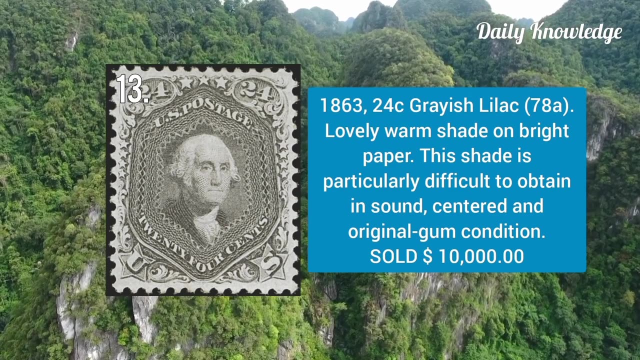 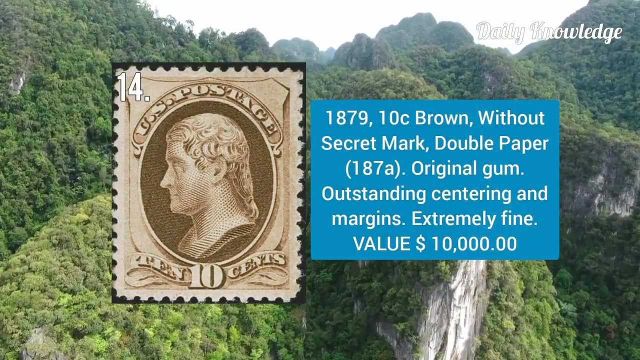 difficult to find in this well-centered condition then very fine, rare, sound, unused example of five cent 1856 issue. it is a stamp which is missing from many advanced collection 1863, 24 cent grayish lilac and it has lovely warm shade on bright paper and it is well centered. 1879, 10c brown, without. 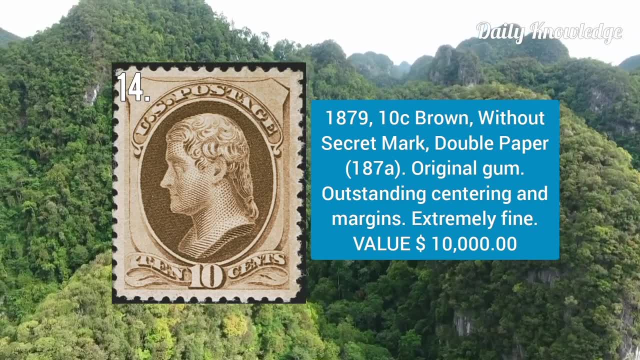 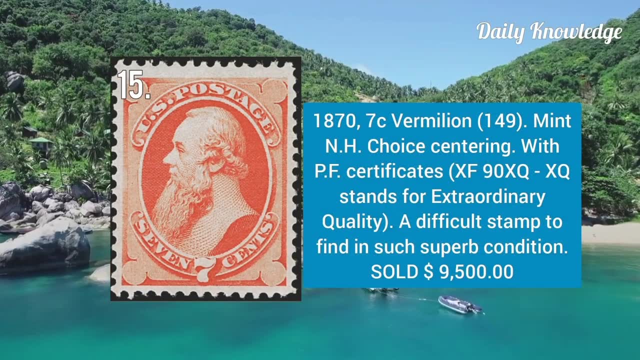 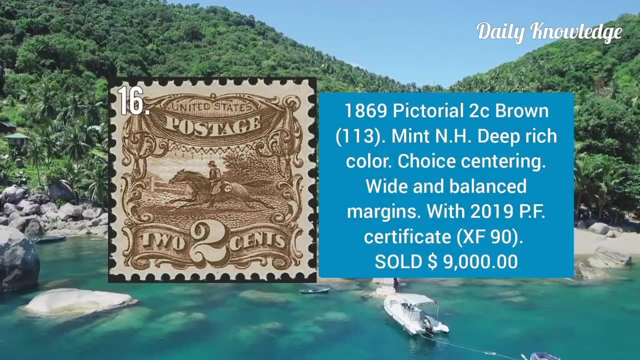 secret mark and it is on double paper. it has original gum and outstanding centering. now, 1877 c vermilion mint, never hinged. it has choice centering with certificate and it is a difficult stamp to find. 1869 pictorial 2 cent brown mint, never hinged. 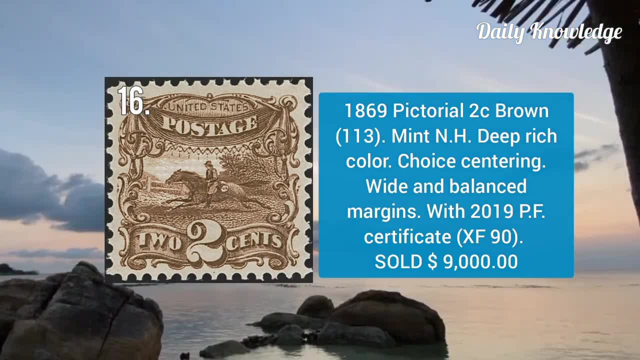 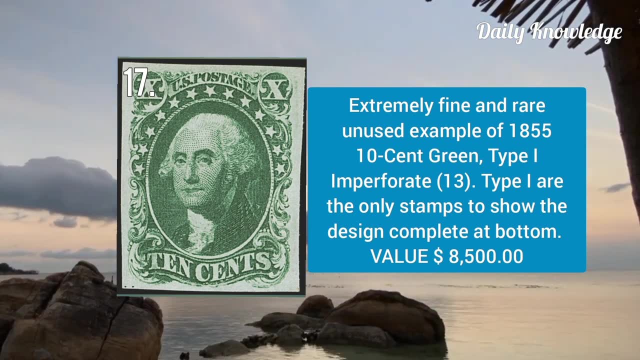 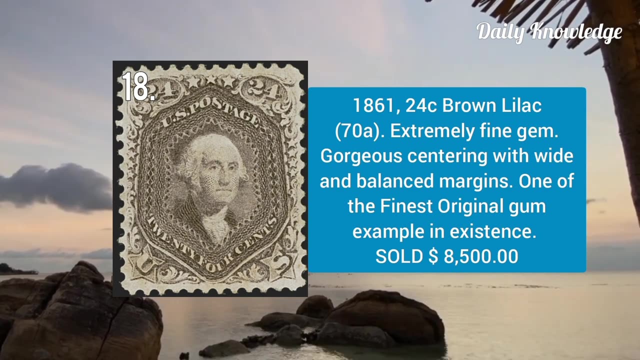 it has deep, rich color choice centering and white and balanced margins. extremely fine and rare unused example of 1855, 10 cent green type 1 in perforated stem and it is a design complete at bottom. 1861, 24 cent brown lilac: extremely fine gem, gorgeous entering. 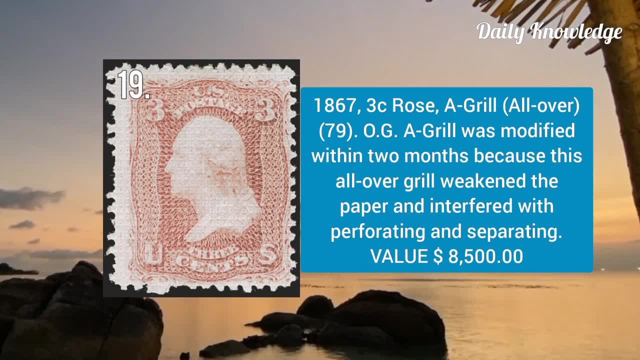 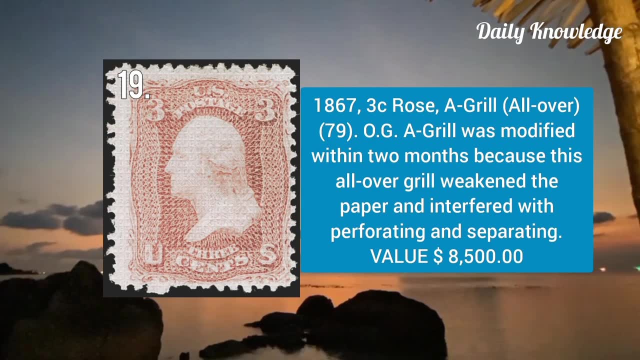 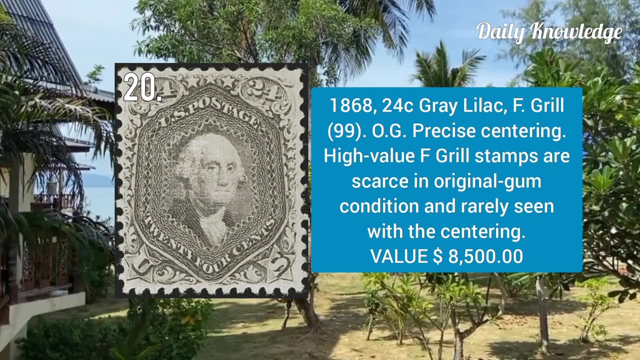 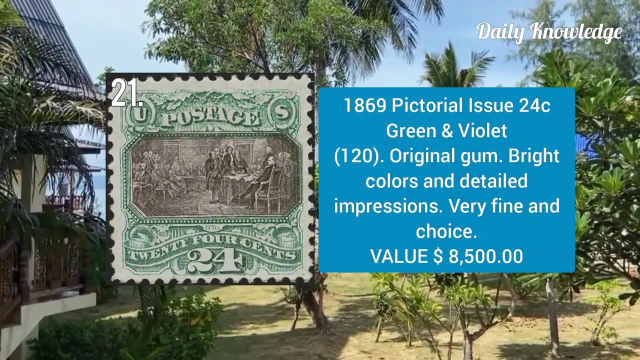 with white and balanced margin and original gum. 1867, 3 cent rose a grill and it has original gum and a grill was modified within two months now. 1868, 24 cent gray lilac f grill. it has original and high value of f grill. stamps are difficult to find. 1869, pictorial issue: 24 cent green and violet. 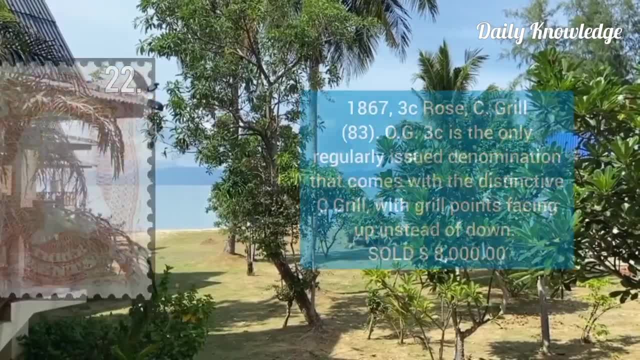 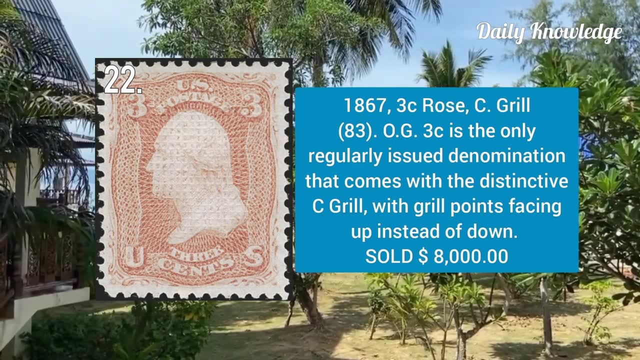 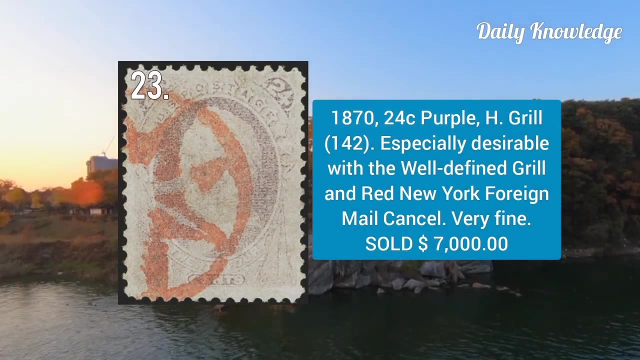 and it has original gum, bright color and detailed impression. this is 1867 three cent rose sea grill with original gum and the grill points are facing up instead of down. next is 1870 24 cent purple h grill, especially desirable with the well-defined grill, and red new york foreign meal cancer. now soldiers, fair stamford, 15 cent pale brown, and these stamps were issued during the fair on july 27 1864.. 1870, 24 cent purple, age grill points up and it has well struck segmented cork cancer and it is fresh and verifying now, 1893. 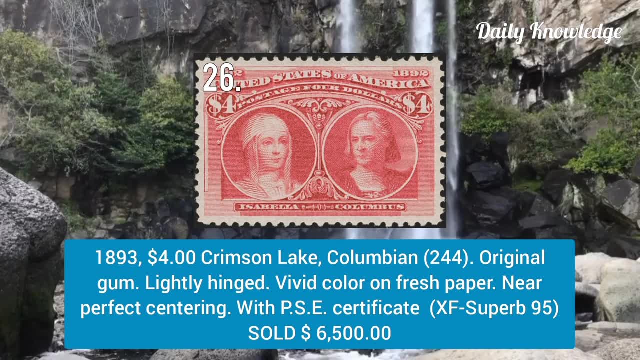 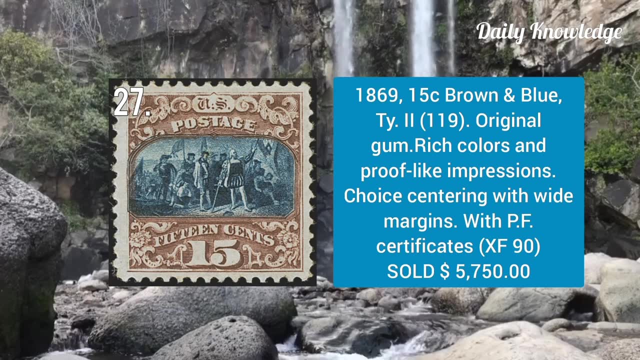 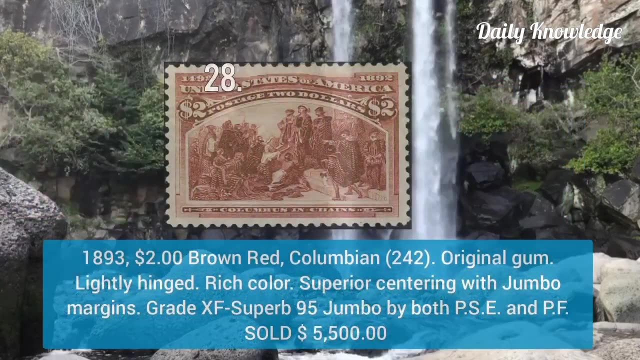 four dollar crimson lake colombian with original gum and it is lightly hinged now. next is 1869: 15 cent brown and blue type 2. it has original gum, rich colors and proof like impression with choice centric. next is 1893: two dollar brown, red colombian issue. it has original gum, rich color. 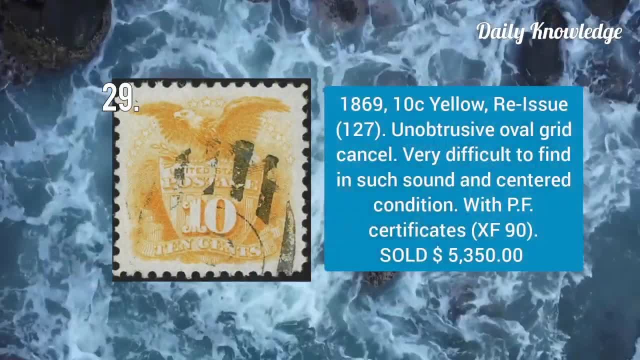 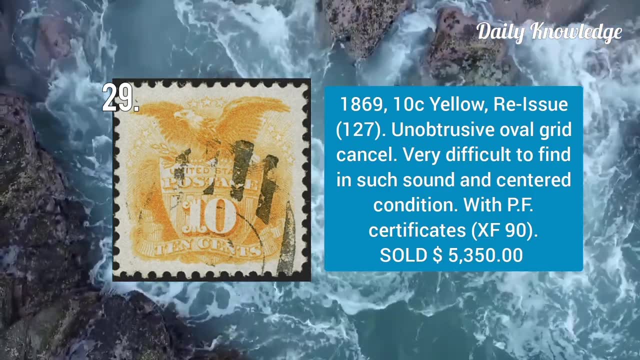 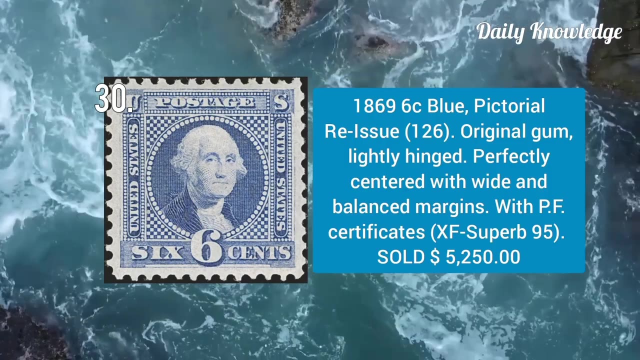 and a superior centering with jumbo margins. 1869 10 cent yellow reissue. unobtrusive oval grid cancel. it is very difficult to find in such sound and centered condition. 1869 6 cent blue pictorial reissue. it has original gum, is lightly hinged and perfect centric with white. 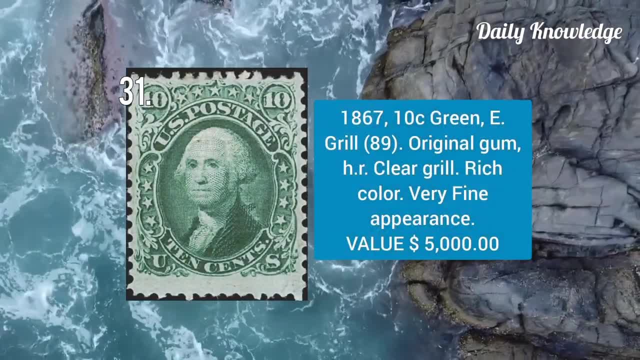 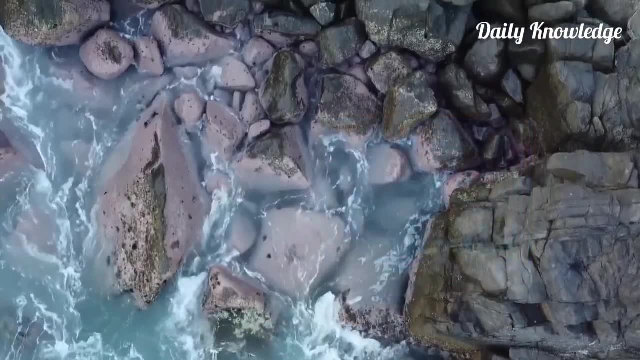 margins. 1867, 10 cent green e grill with original gum and clear grill. it has original gum, rich colors and proof like impression with choice and proof like impression with rich color and very fine appearance. next is 1861, 15 cent black, with original gum detailed. 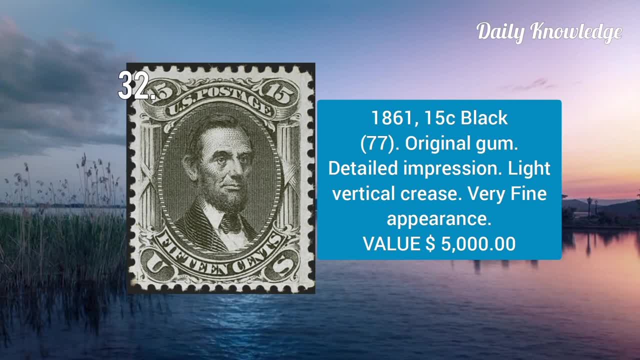 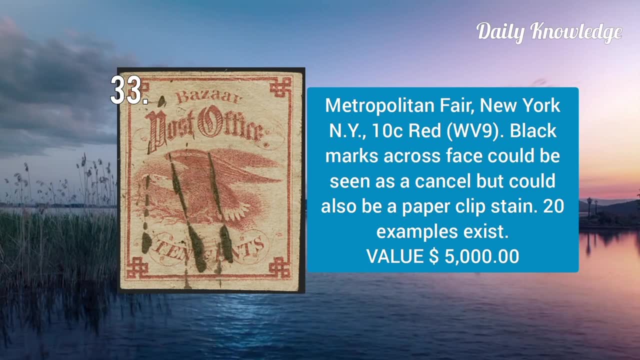 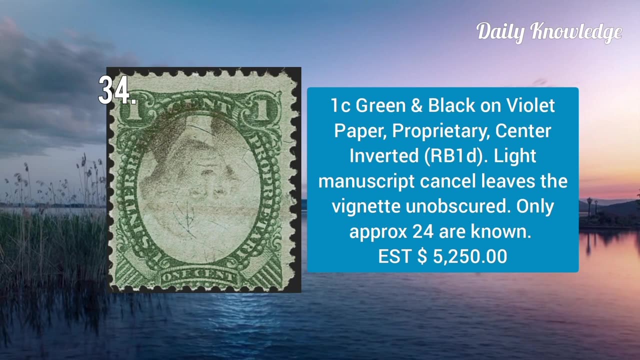 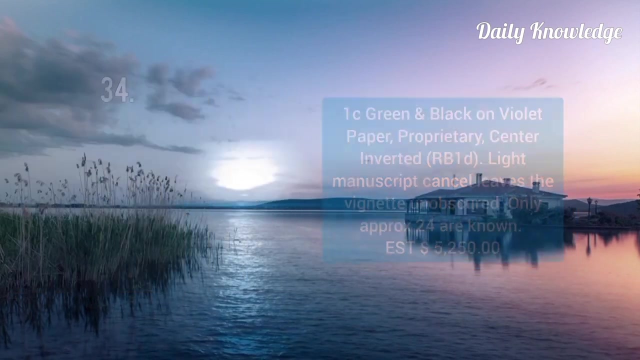 impression and his light vertical crease. otherwise it is very fine. now metropolitan fair, new york: 10 cent red color, black marks across the face and these are seen as cancel. now one cent green and black on violet paper propriety issue and center is inverted. it has light manuscript cancel. next is philippines, 1903. two dollar dark blue block of four with 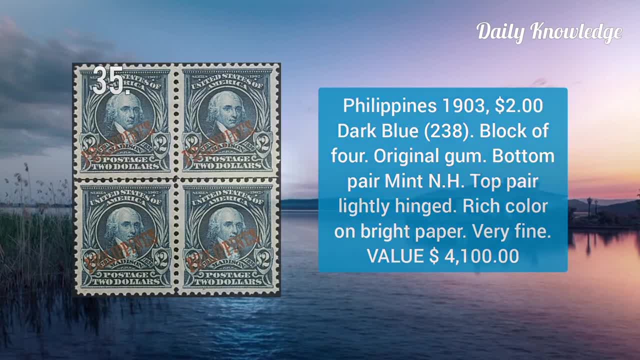 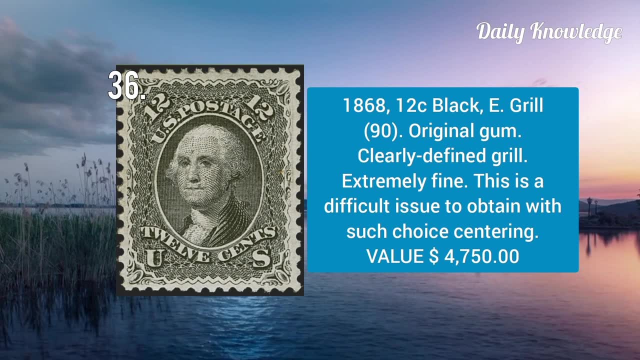 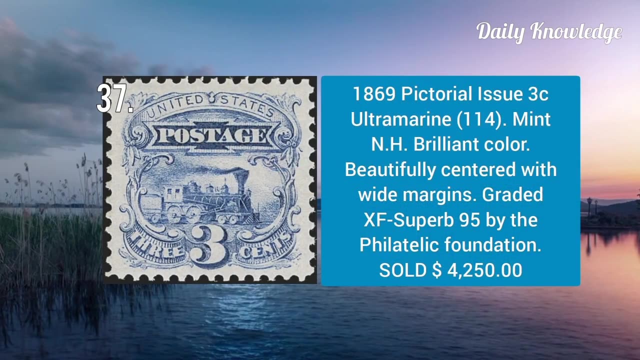 original gum and bottom pair is mint, never hinged, and it is very fine. 1868 12 cent black e grill with original gum, clearly defined grill, and it is extremely fine and it's very difficult to find. next is 1869 pictorial issue: three cent ultra made in. it is mint, never hinged. 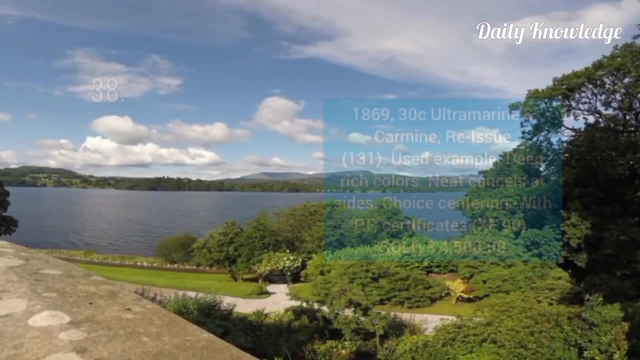 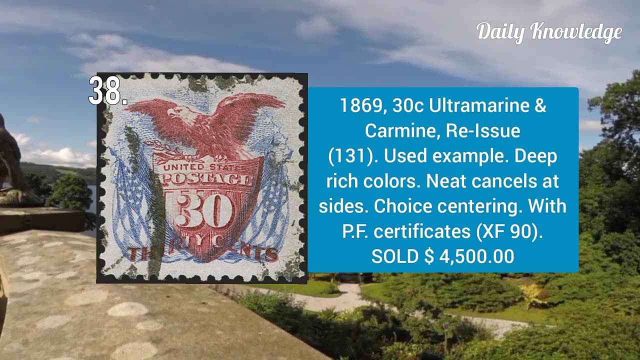 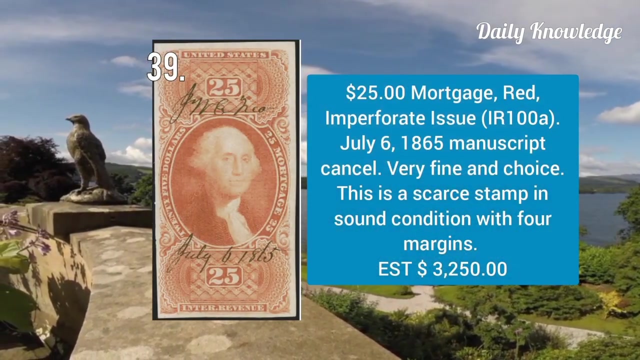 is brilliant color and white margins. 1869 30 cent ultramarine and carmine reissue used example with deep, rich color and neat cancel at the sides. this one is 25 dollar mortgage read in perforate tissue and has manuscript cancel and is very fine and twice it is a scar stamp in sound condition. 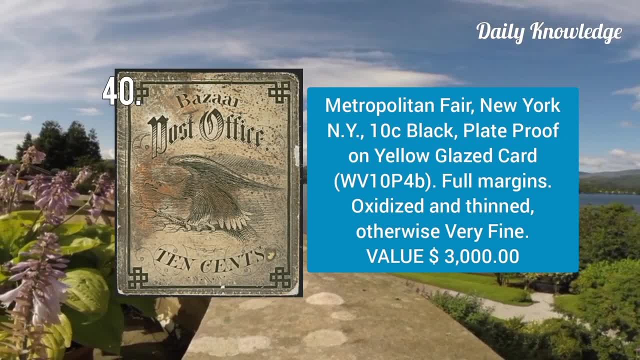 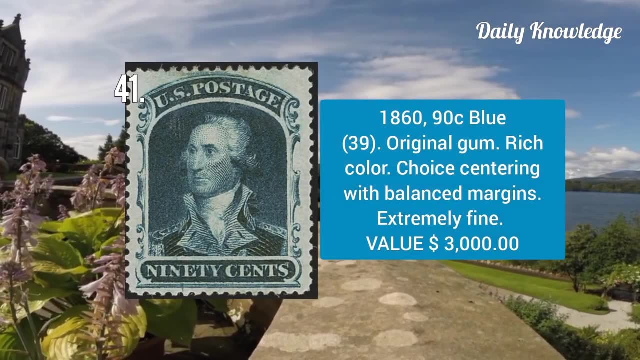 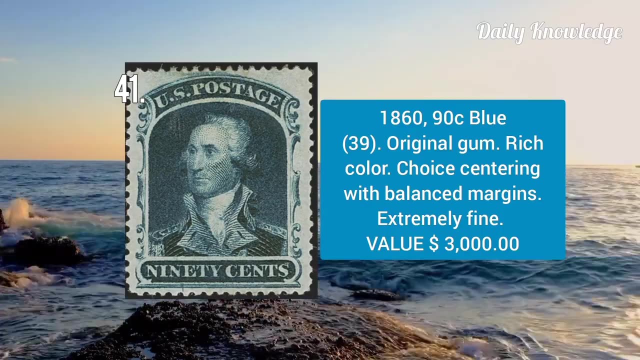 Metropolitan Fair, New York. ten cent black plate proof on yellow glazed card. it has full margins and is oxidized and thin. 1860, 90 cent blue with original gum, rich color choice, centering and balanced margin and it is extremely fine. next is 1867, one cent blue, e-grill. 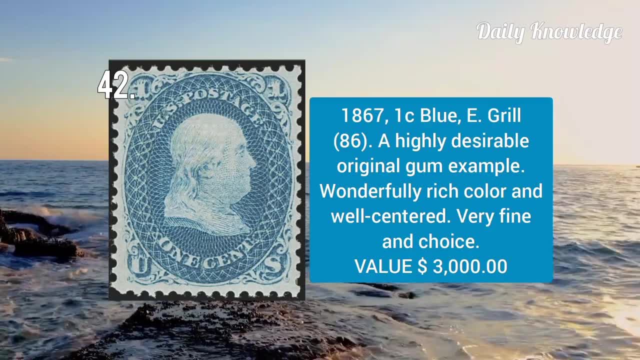 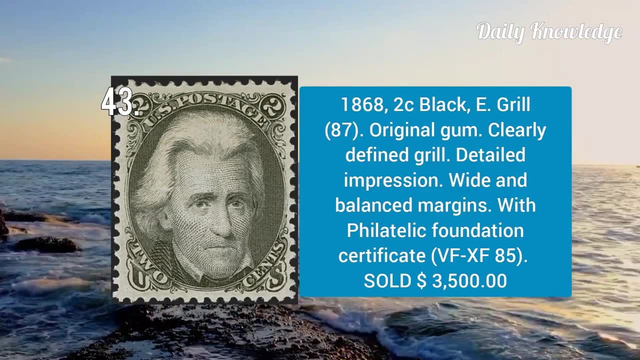 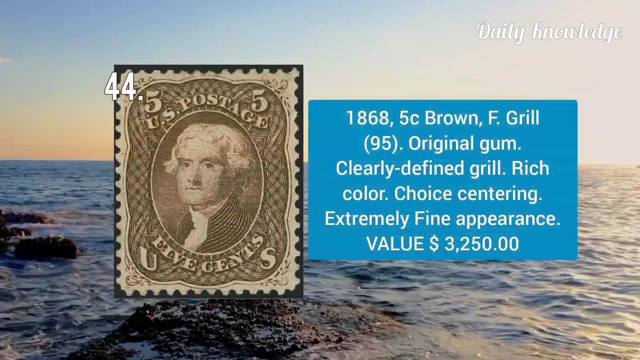 it is a highly desirable original gum example and has wonderful rich color and is well centered. 1868 2c black e-grill with original gum, clear, detailed grill and detailed impression. it has white and balanced margin and is extremely fine. 1868 5 cent brown f-grill with original gum and. 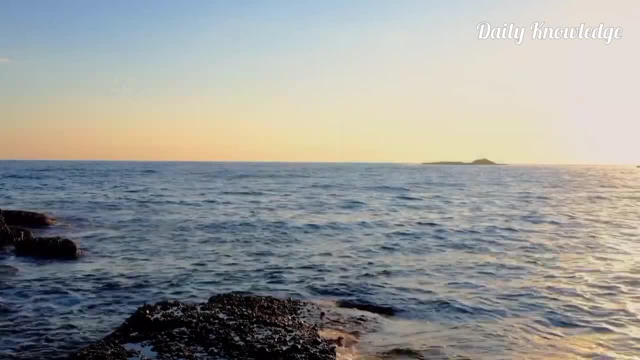 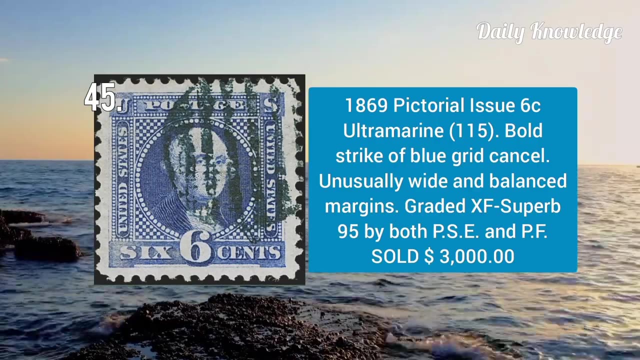 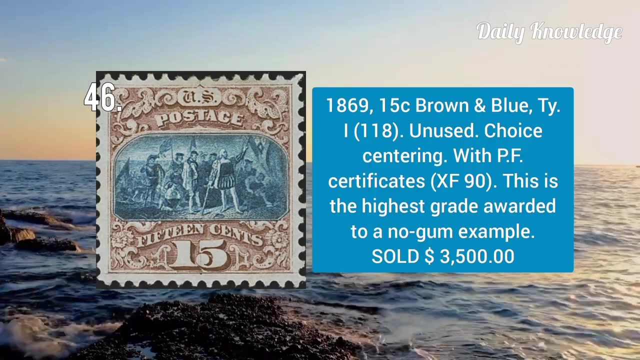 clearly defined grill. it has rich color and has choice centering. 1869, pictorial issue: 6 cent ultramarine with bold strike of blue grit cancel. it has unusually white and balanced margins. 1869, 15 cent brown and blue type 1. it is unused and has choice centering. it is graded. 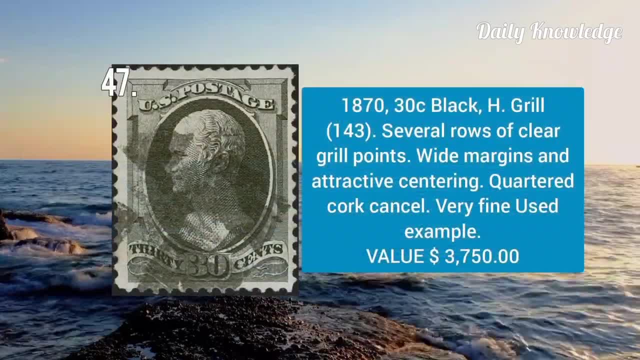 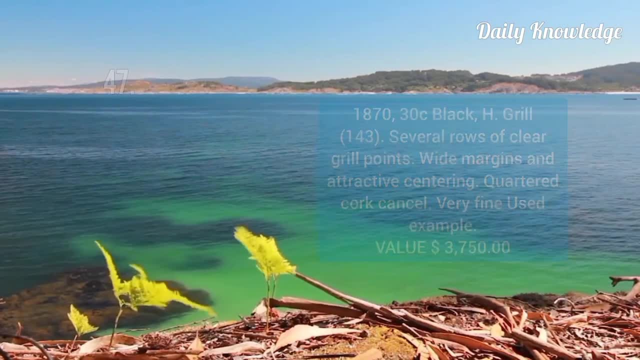 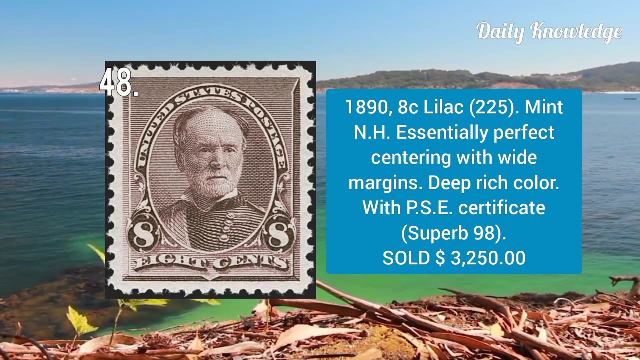 extremely fine. 90 now 1870, 30 cent black h grill, several rows of clear grill points. it has white margin and attractive centering. now this is 1898 cent lilac mint, never hinged. it has perfect centering with white margin and has a deep, rich color. 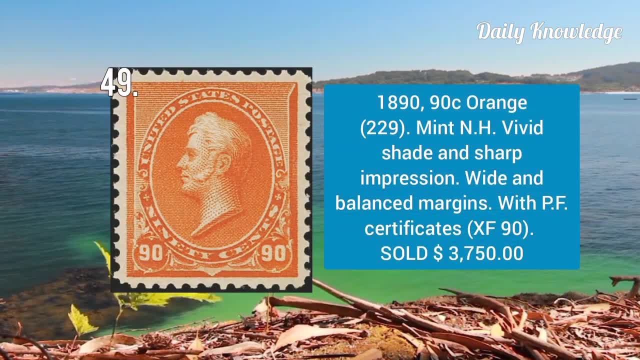 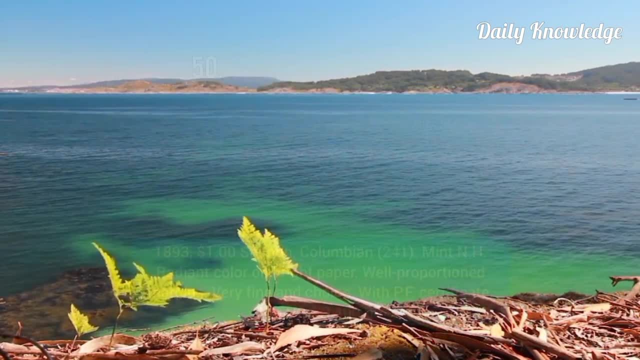 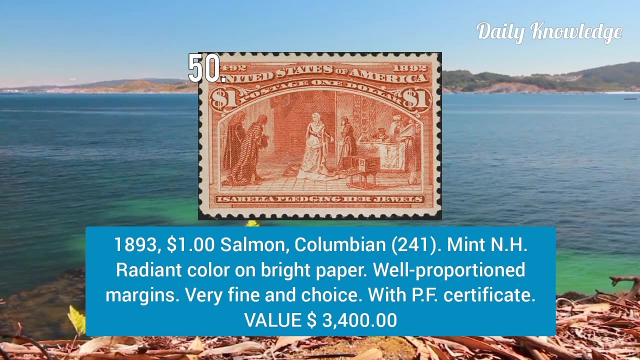 now this one is 1890, 90 cent orange mint, never hinged, and has vivid shade and sharp impression. it has white balanced margin and is extremely fine. 1893, one dollar salmon columbian issue mint, never hinged. it has radiant color on bright paper and is well proportioned. 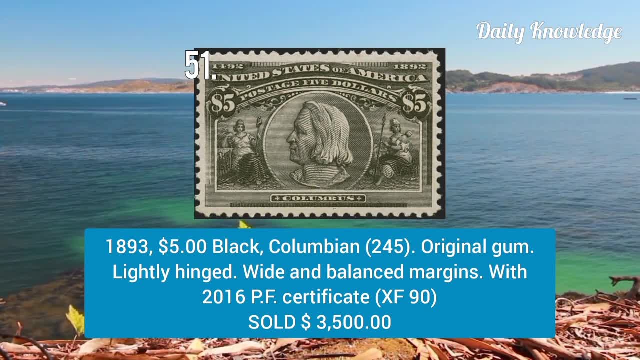 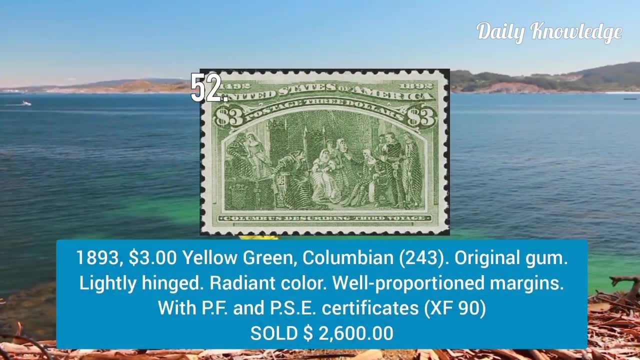 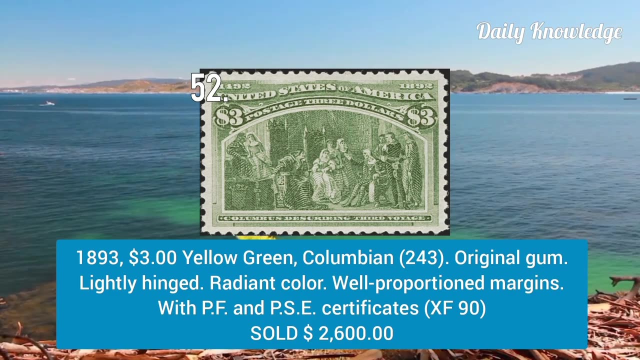 next is 1893. five dollar black columbian issue and it has original gum. it is lightly hinged and is white and balanced margin. this is 1893. three dollar yellow green columbian issue. it has original gum, printed color, well proportioned margins and is lightly hinged. six cent brown red mint, never hinged with. 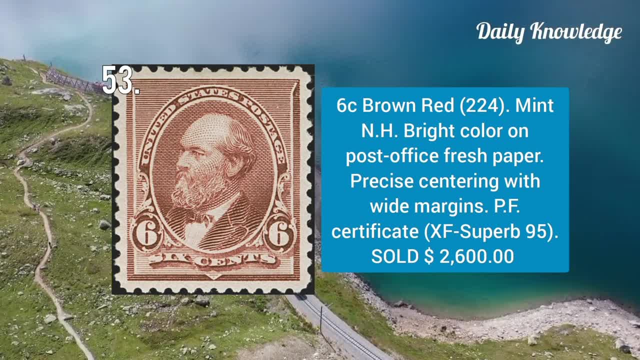 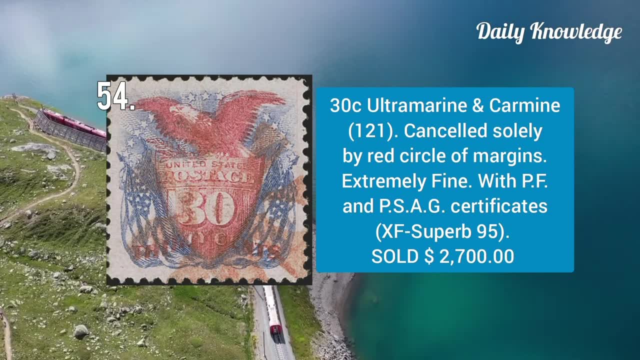 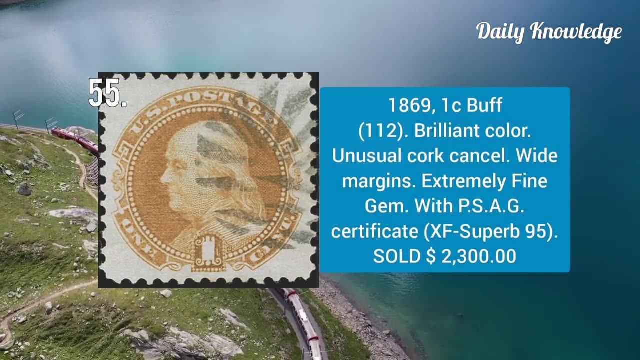 bright color on post office fresh paper. it has precise centering with white margins. next is 30 cent ultramarine and carbine. it is cancelled solely by red circle of margins and it is extremely fine. it is accompanied with philatelic certificate 1869. one cent buff, brilliant color, unusual cork cancel. 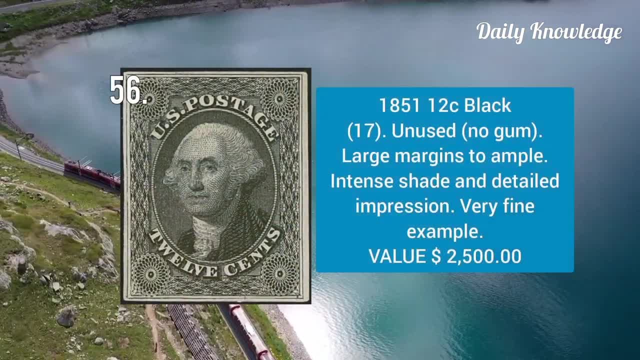 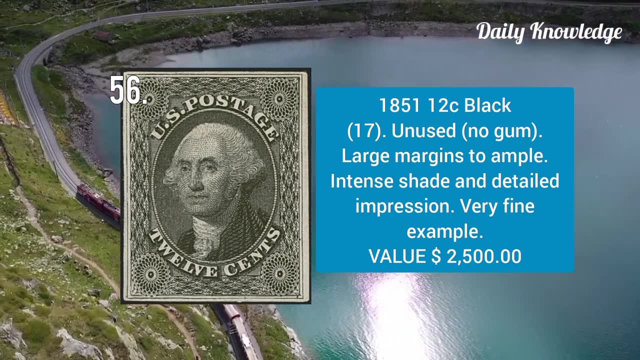 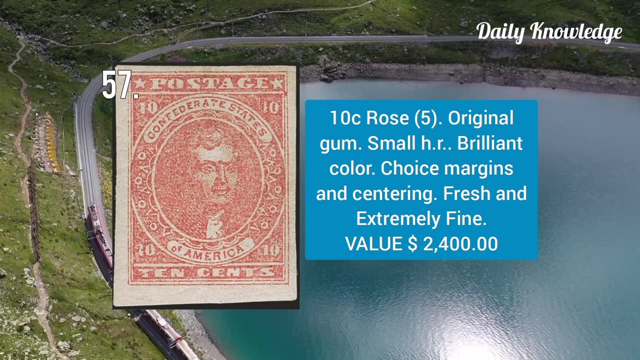 and white margins and it is extremely fine. gem 1851, 12 cent black, unused with no gum and it has large margins to ample, intense shade and detailed impression. 10 cent rose, original gum, small hinge remnant and it has brilliant color choice, margin and centering and it has a large margin and it has. 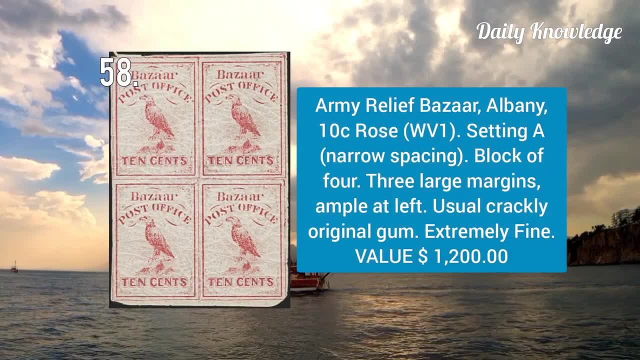 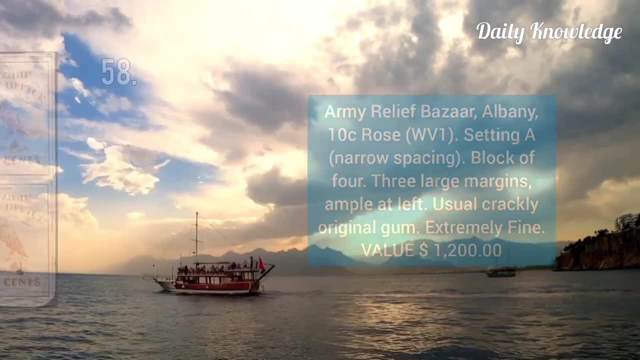 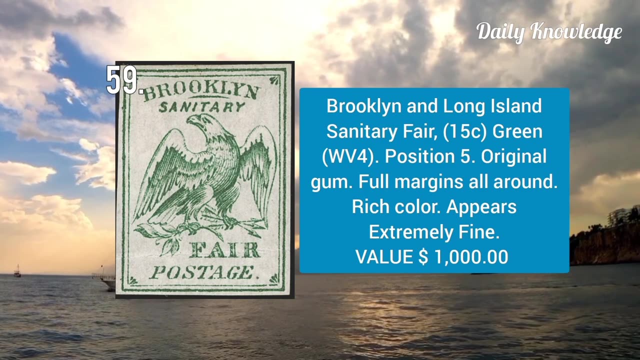 it is fresh and extremely fine. next is army relief bazaar: albani: 10 cent rose, setting a narrow spacing block of four and three large margins. brooklyn and long island sanitary fair: 15 cent green position five with original gum, full margins all around and rich color. 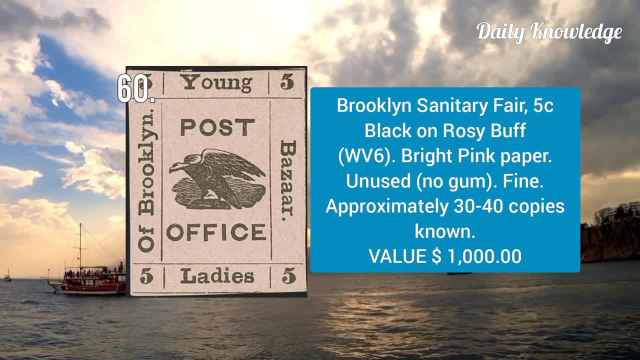 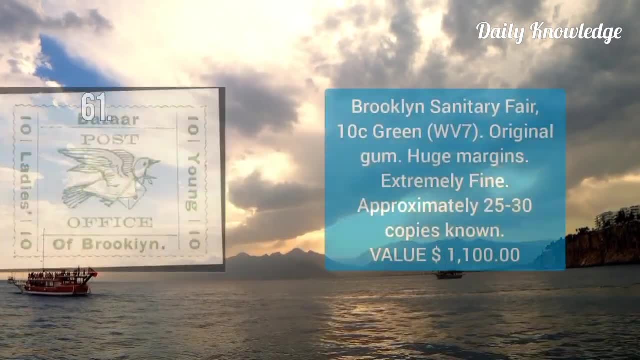 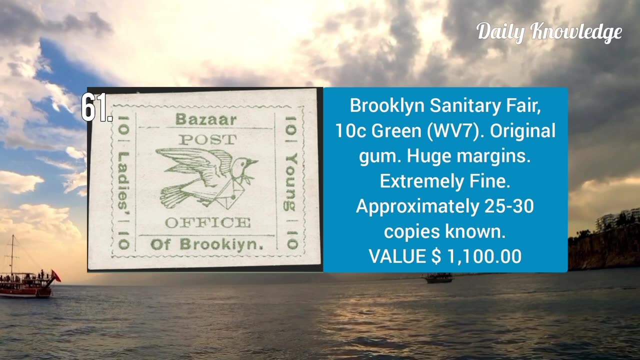 now. brooklyn sanitary fair: five cent, black on rosy buff and it is on bright pink paper. it is unused with no gum. only 30 to 40 copies exist. brooklyn sanitary fair: 10 cent: green with original gum, huge margins. it is extremely fine and only 25 to 30 copies. known canal zone 1904. eight cent. 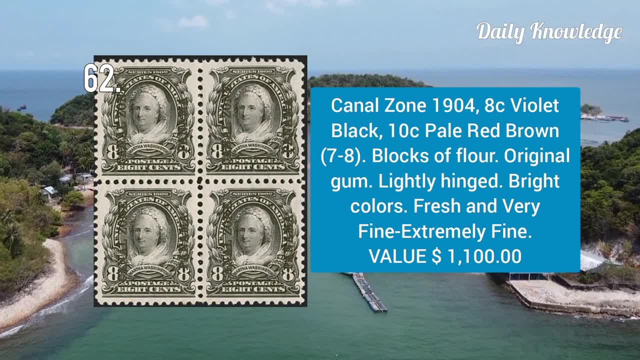 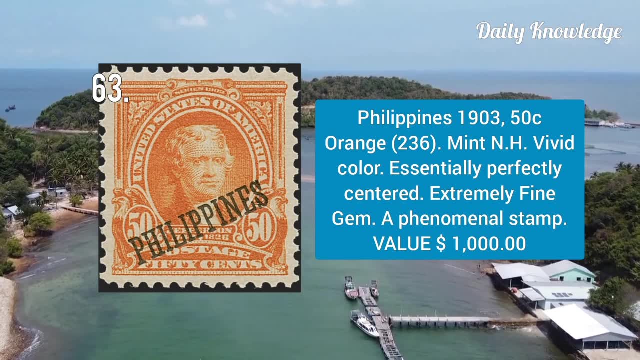 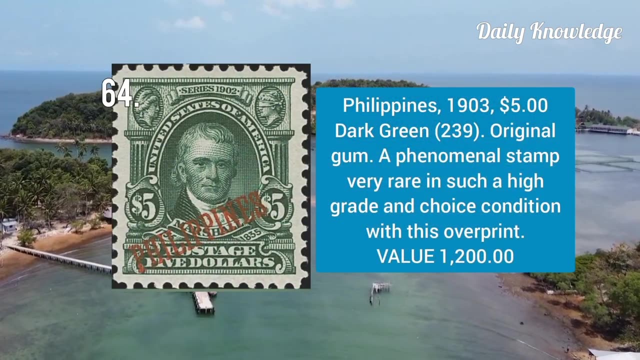 violet, black, 10 cent. pale, red, brown block of four. it is with original gum and is lightly hinged. philippines 1903- 50c. orange mint, never hinged, it has vivid color and has perfect centering and it is extremely fine now. philippines 1903- five dollar. dark green. 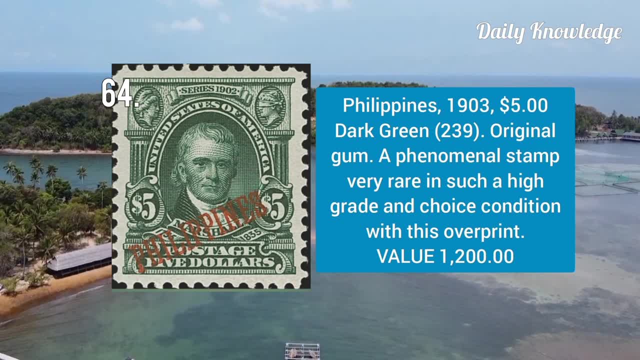 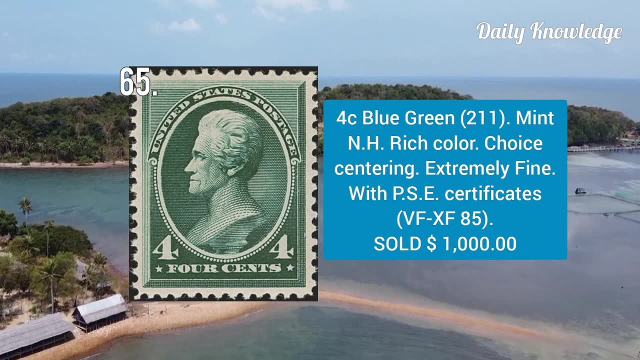 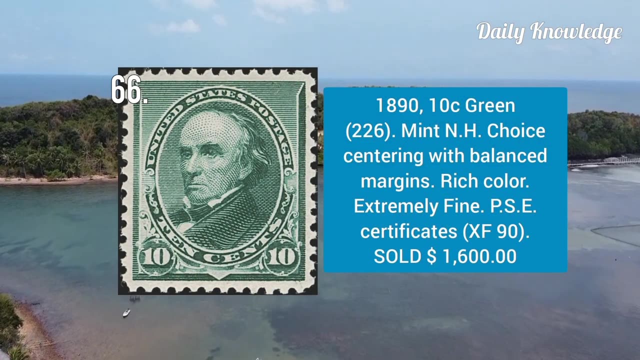 with original gum. it is a phenomenal stamp and is very rare to find in such choice centering. four cent blue green mint, never hinged, with rich color, choice, centering and extremely fine, and it is accompanied with philatelic certificate. now, 1890, 10 cent green mint, never hinged, choice. 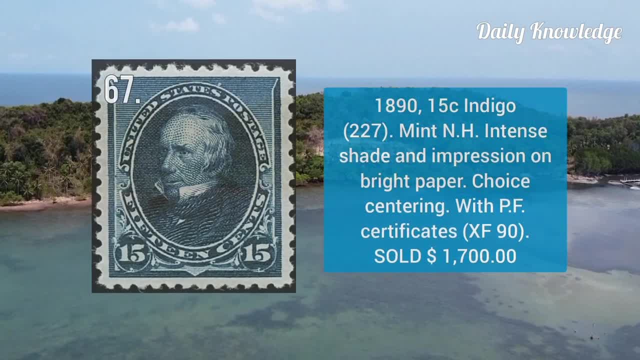 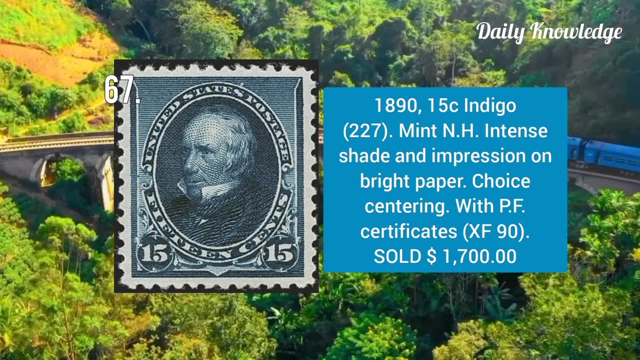 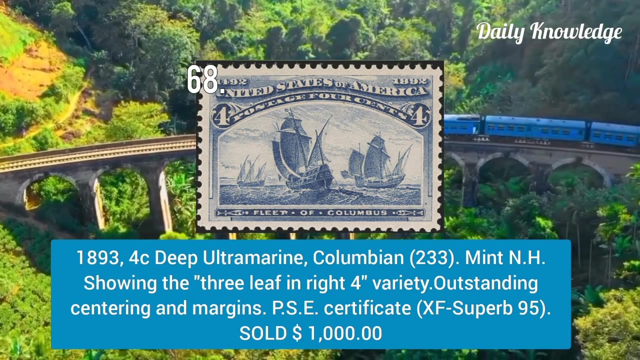 color and it is also accompanied with philatelic certificate. this is 1890 issue, 15 cent indigo mint, never hinged, with intense shade and impression on bright paper, and it has choice centering 1893, four cent deep ultramarine columbian issue. it is mint, never hinged and is showing the three leaf in 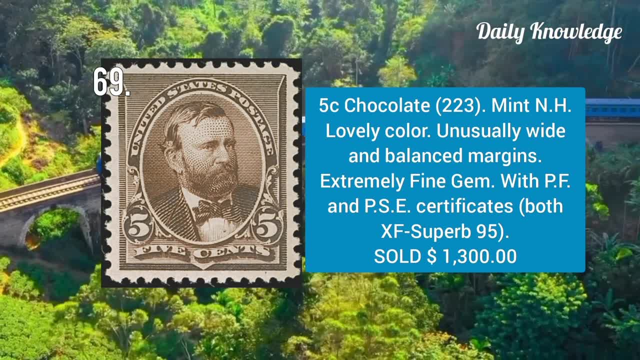 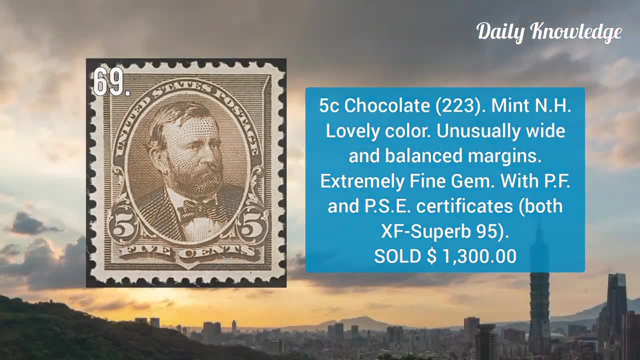 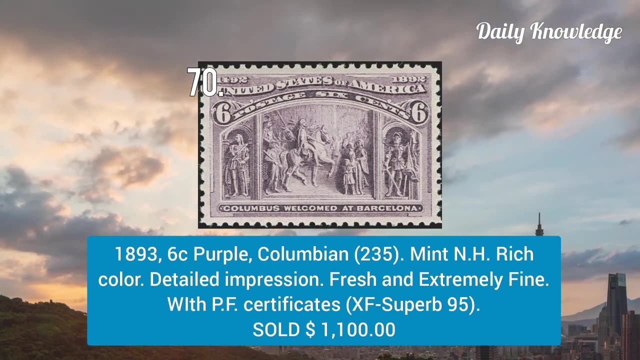 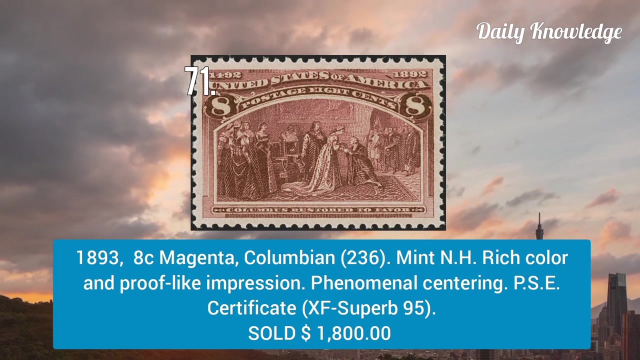 right four variety. then five cent chocolate mint, never hinged, with lovely color and it has unusually balanced margin and it is extremely fine. 1893, six cent: purple columbian issue mint, never hinged, with rich color, detailed impression, and it is fresh and extremely fine. next is 1890: three eight cent. 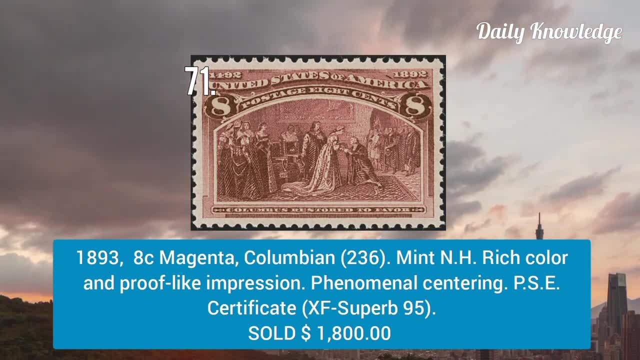 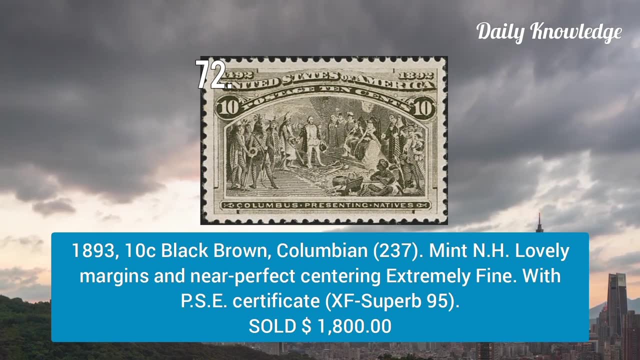 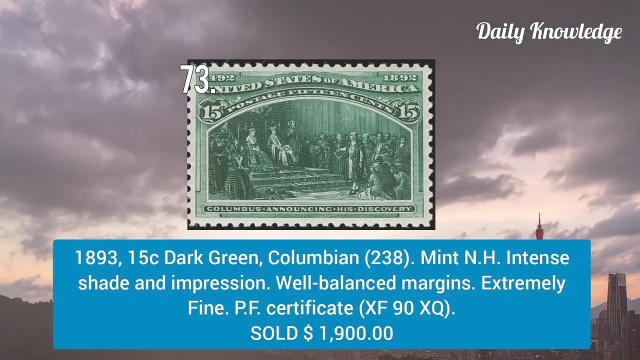 magenta columbian issue and it is also mint, never hinged, with rich color and proof like impression. now next is 1890, three 10 cent black brown columbian issue. it is also mint, never hinged margins and near perfect centering and is extremely fine. 1893, 15 cent dark green columbian issue mint. 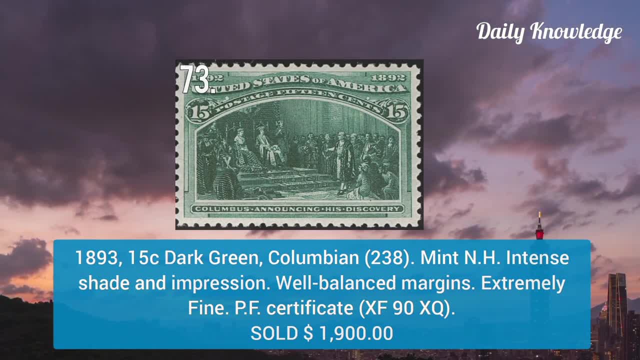 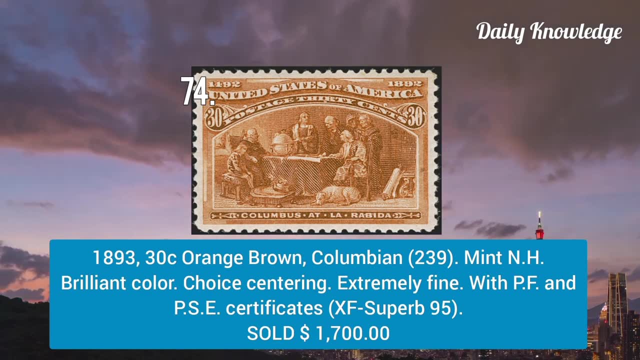 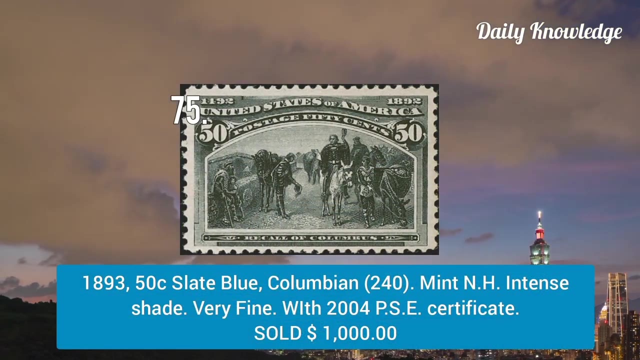 never hinged, with intense shade and impression. it is extremely fine. 1893, 30 cent orange, brown columbian issue mint, never hinged, brilliant color choice, centering, extremely fine and it is superb. 95 graded. 1893, 15 cent slate blue columbian issue mint, never hinged, with intense shade and 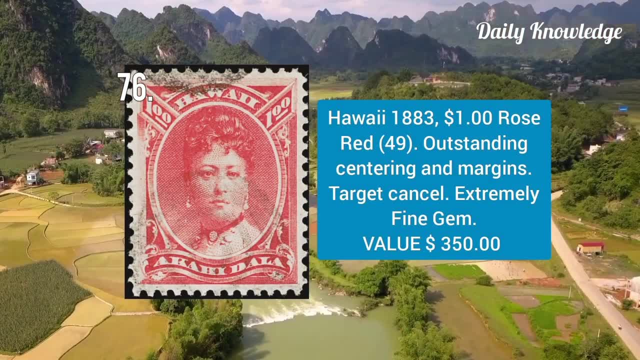 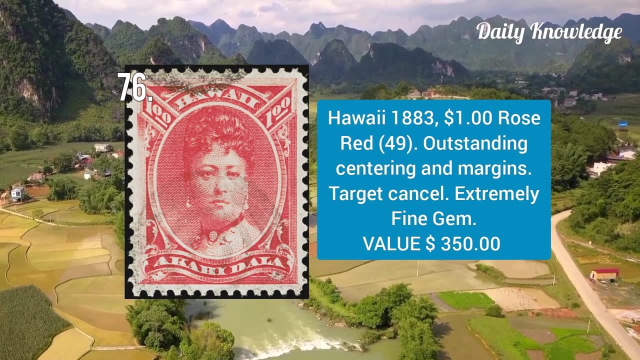 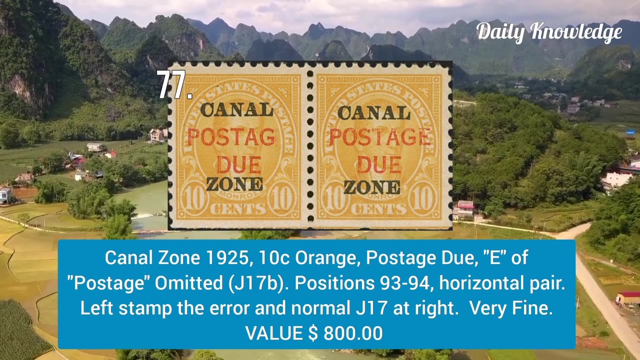 very fine appearance. next stamp is from hawaii 1883, one dollar: rose, red, outstanding centering and margins target cancer and it is extremely fine. gem canal zone 1925, 10 cent orange postage due. e of the postage is omitted and is position 93 to 95. 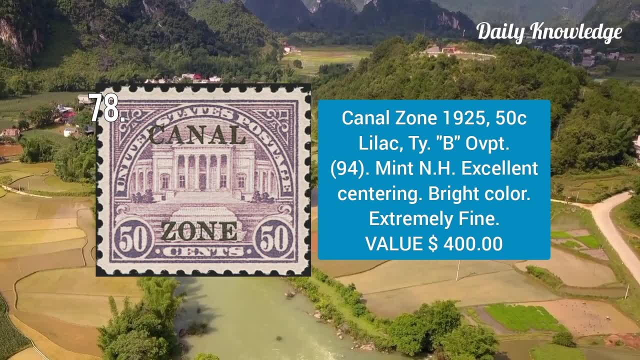 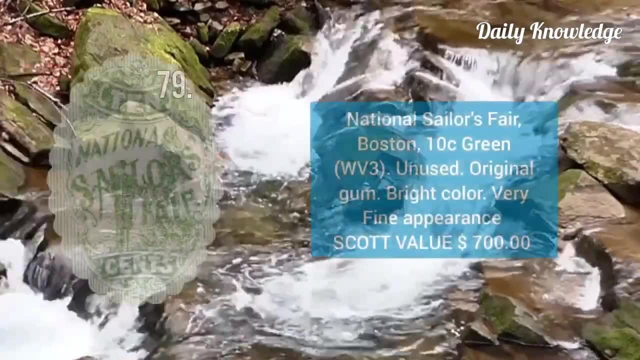 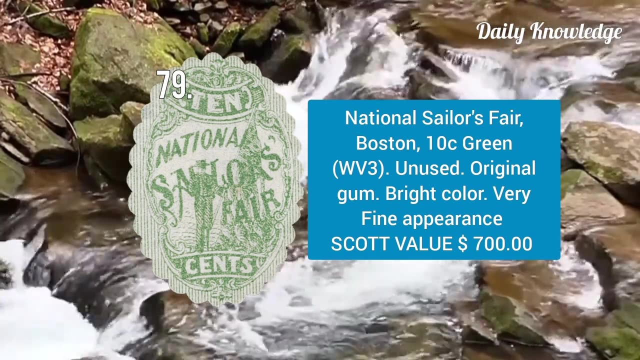 horizontal pair can also: 1925, 50 cent lilac type b overprint. it is mint, never hinged and has excellent centering and bright color. national sailors: fair boston, 10 cent green, unused with original gum, bright color and very fine appearance. now next is great central fair philadelphia, 20. 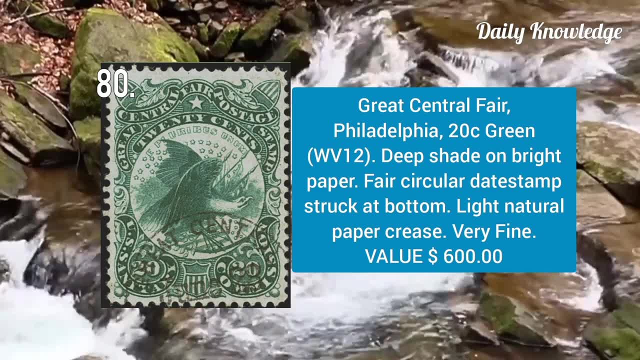 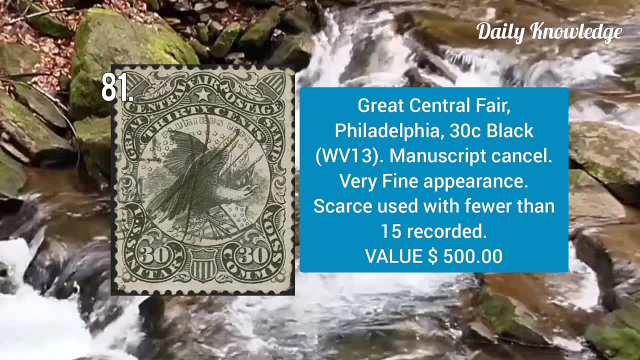 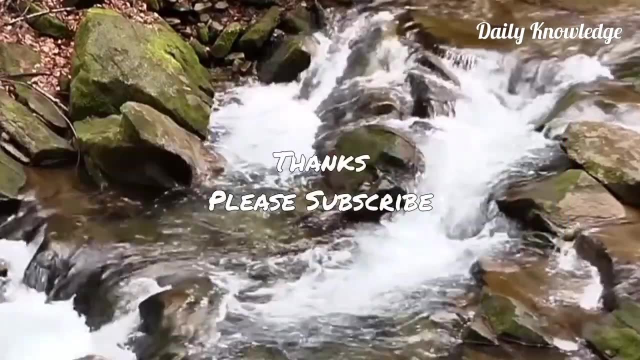 cent green deep shade on bright paper and fair circular date stamp. stock at the bottom: you, and it is very fine. great central fair philadelphia. 30 cent black manuscript cancel. it has very fine appearance and only 15 examples recorded. okay, friends, thanks for watching. please like share. comment and subscribe to my channel.